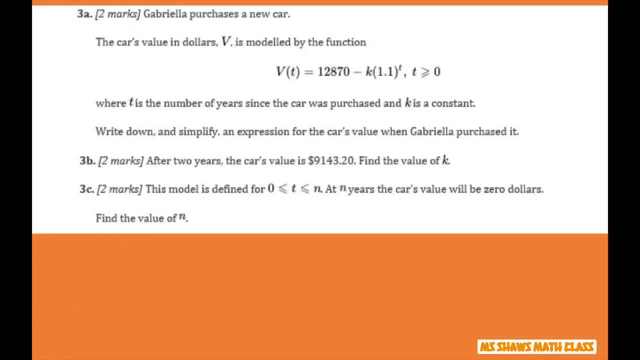 Hi everyone. Gabriela purchased a new car. The car's value in dollars fee is modeled by the given function. T is the number of years since the car was purchased and K is a constant Write down and simplify an expression for the car's value when Gabriela purchased it. 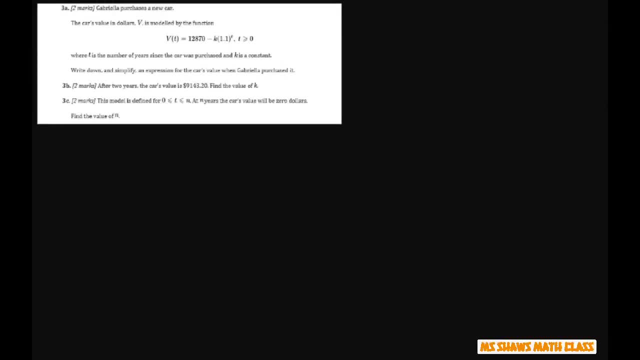 So basically, what they want is, at time, zero. what was the purchase of the car? So basically, you're going to write 1, 2, 8, 7, 0 minus K times 1.1 to the zero power. 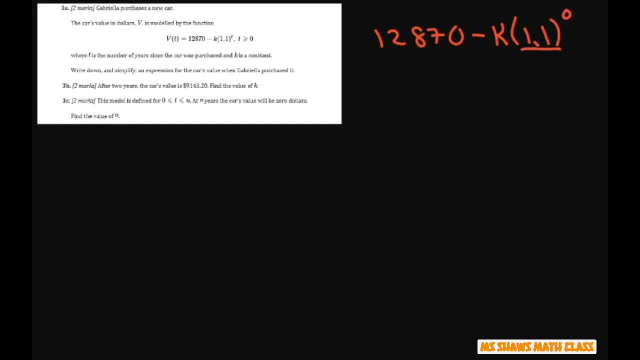 Now that's just going to be 1.. This part's 1.. So your answer is 1,, 2,, 8.. 7, 0 minus K. Now it says: after two years, the value is this amount. Find the value of K. 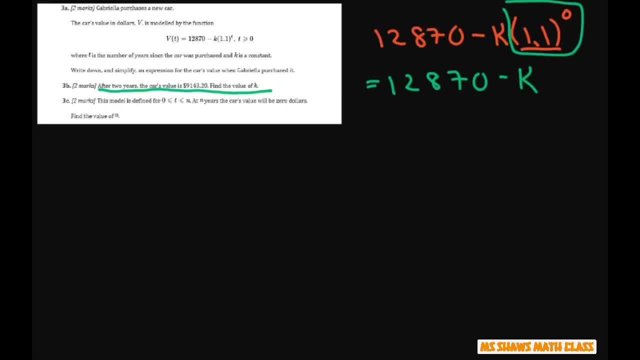 So all you're going to do is plug in your formula. here We have 9,143.20 equals 12,870.. Minus K times 1.1 squared. So simplifying all that we subtract, Let's see: 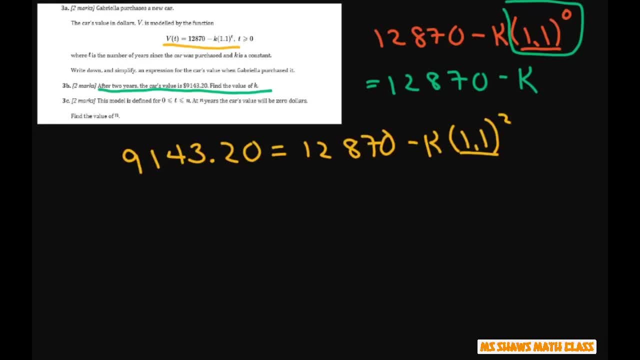 We can square that. Let's subtract, You get 9,143.20 minus 12,870, and this gives you negative 3,726.8 equals negative K and 1.1, let's see 1.1 squared. 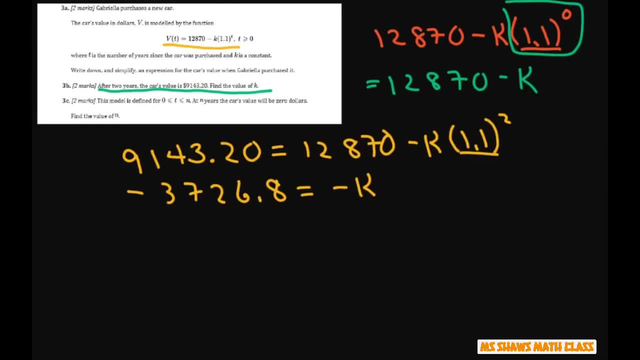 Oops, I forgot to put my parentheses. That's going to be K, So the solution is going to be minus. Let's write it like this: Minus 1.21K. So divide both sides by negative 1.21.. 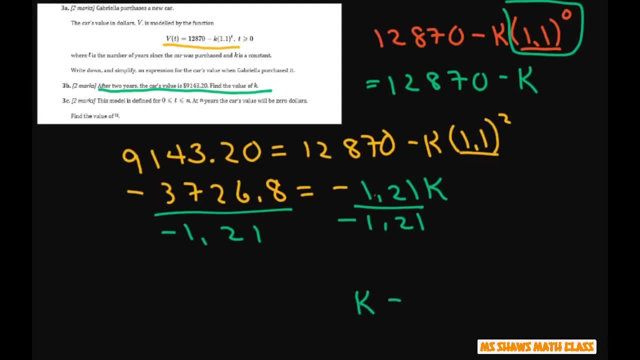 And you'll get K equals 3,080.. Now you get minus 1.21.. That's going to be minus 1.21.. That's the answer. So if you do that, you're going to see 1.21, that's going to be minus 1.21.. 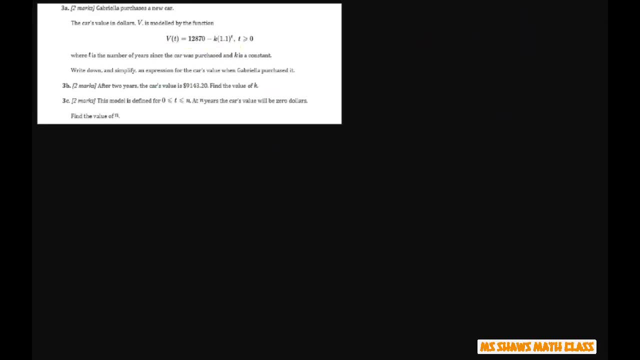 And then you add that Now it says this model is defined for time between 0 and N. After N years the car's value will be $0.. Find that value. So basically we're trying to solve for N. 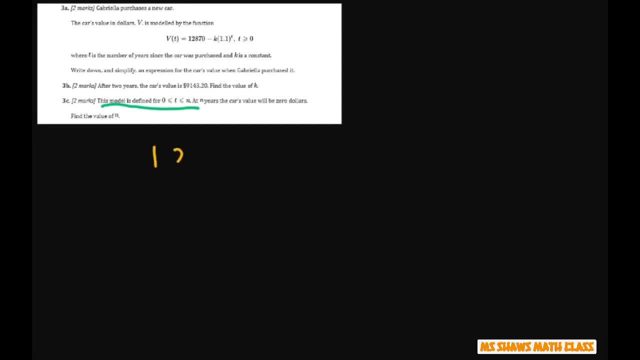 So what you do is you write 1,, 2,, 8,, 7,, 0 minus. your K was 3,080 times 1.1 to the N power, And we want the value to be 0. So follow through and substitute. 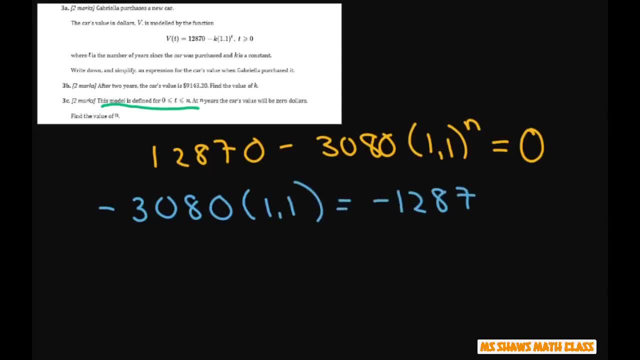 So we get negative 1, 2, 8,, 7, 0.. And this is to the N And divide both sides by negative 30, 80.. So you're going to get- that's going to be positive- 1, 2, 8, 7, 0.. 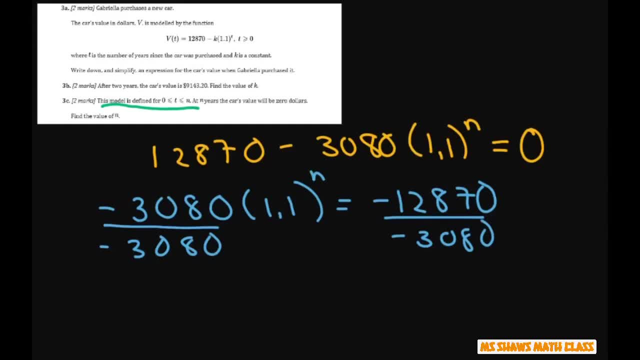 Divide it up 30,, 80. And you're going to get 1.1 to the N power equals 4.1785.. And write out: It's nice, You're going to get as much as you can, Okay. 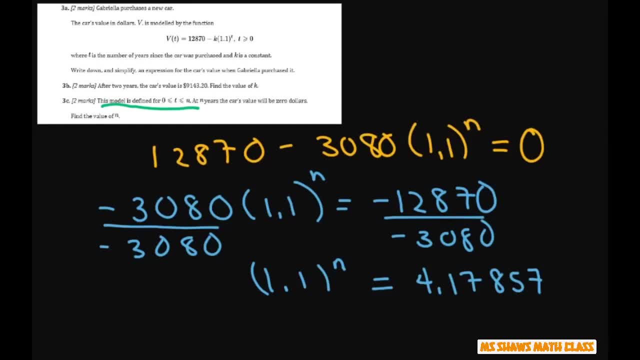 Just to get more of an exact answer. So now you take LN of both sides, You're going to get N times LN of 1.1 equals LN. I did the power property. You take LN of both sides, LN of 4.17857..